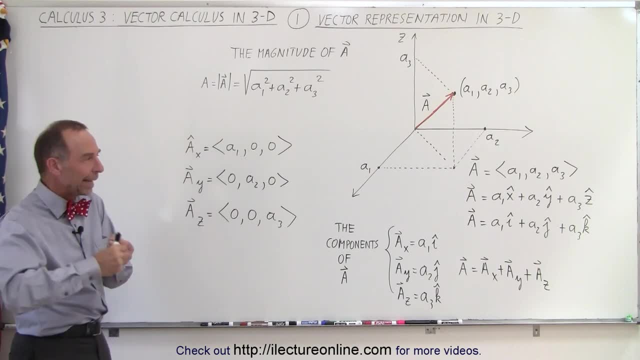 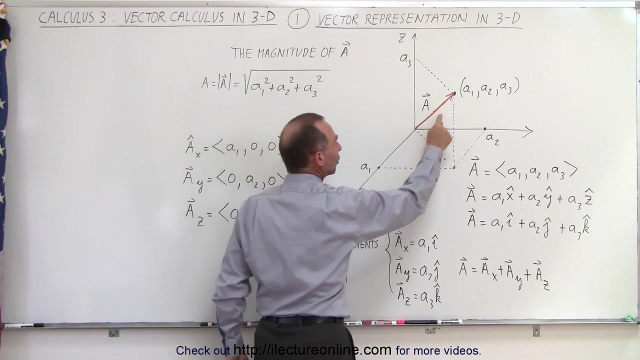 have three components: an x component, a y component and a z component. and in mathematics we often talk about the i, j and k components, which are synonymous to x, y and z. So here we have a point in space some distance away from the origin and the location of that point in space. 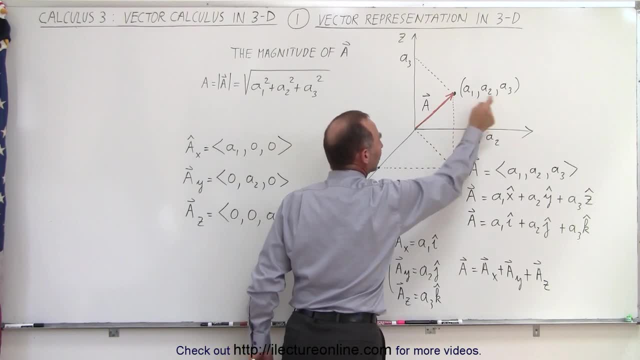 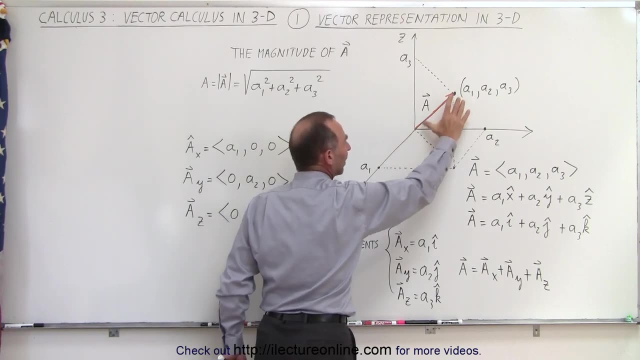 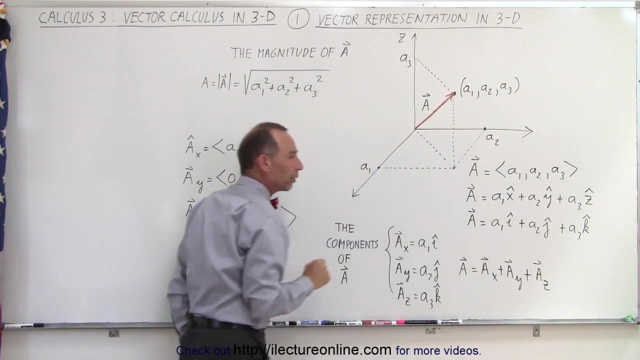 can have the components a1,, a2, and a3.. Now we can define a vector which is a line that starts from the origin and ends at that point, and this would be the length of that vector, and then it would be pointing into that direction, from the origin to that particular point. So we'll talk. 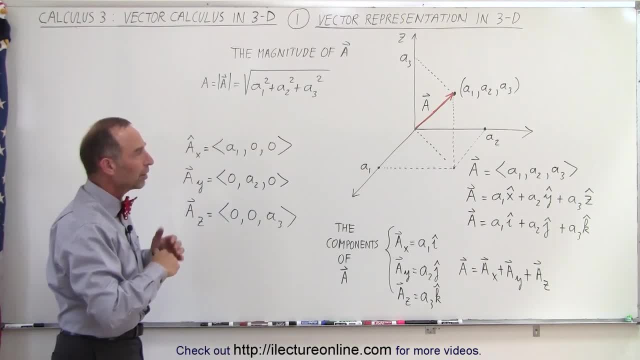 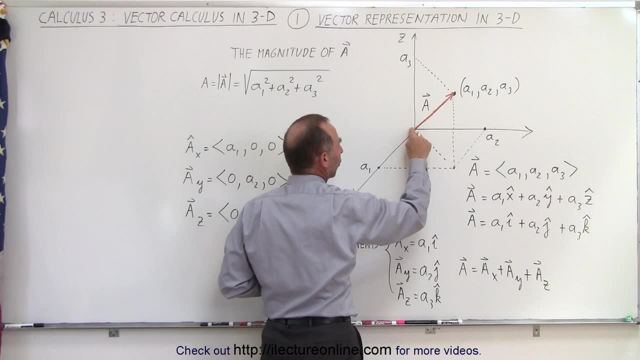 a little bit more about direction of vectors later. Now you can see that the x component here, a1, has a magnitude or length. a1, that's a distance on the origin to the point where this is projected onto the x-axis. project is onto the y-axis then. 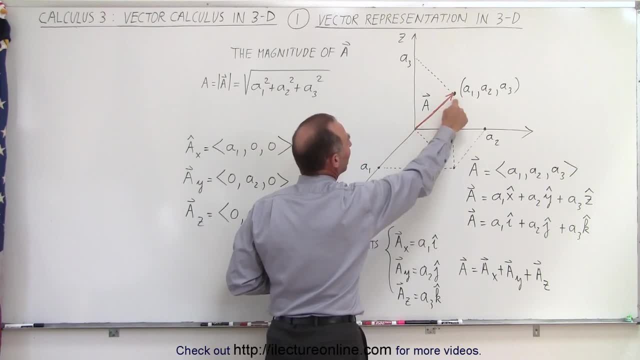 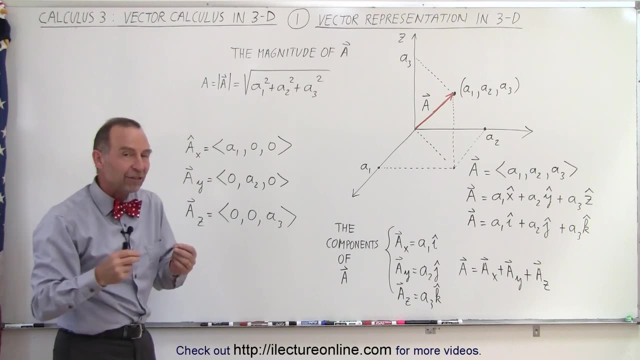 we have a point that's a2 away from the origin and project onto the z-axis where a distance a3 away from the z-axis, and that's how that point is defined. Now we have different ways of notating a vector in three dimensions. we can write the: 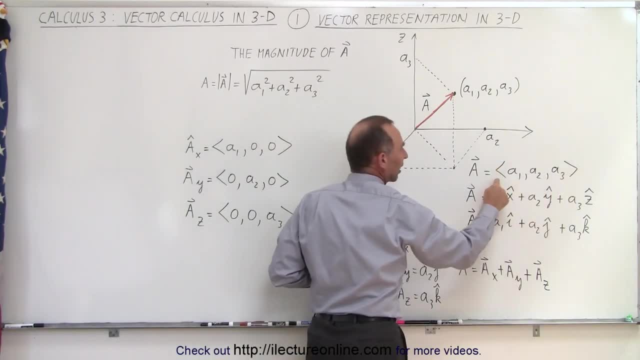 vector a like this, with the two brackets on it on either side, and then the three components of the point that it's pointing to relative to the origin. We can also write it like this: where we have unit vectors x, unit vector, y, unit vector, z, unit vector- and we'll define those later- and then the three component. 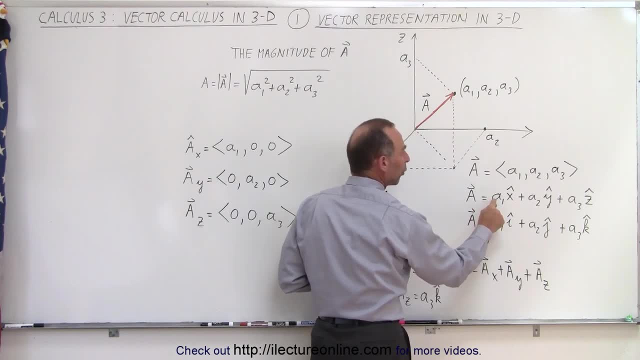 values or magnitudes, the distance from the origin to the point on the x-axis, the distance the origin to the point on the y-axis, the distance from the origin to the point on the z-axis, and those are then the three components of the vector a, or we can, instead of using x, y, 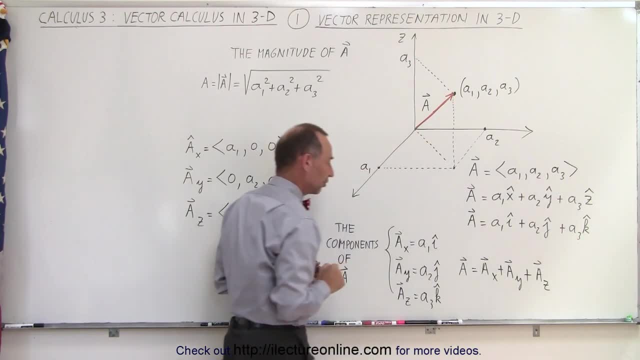 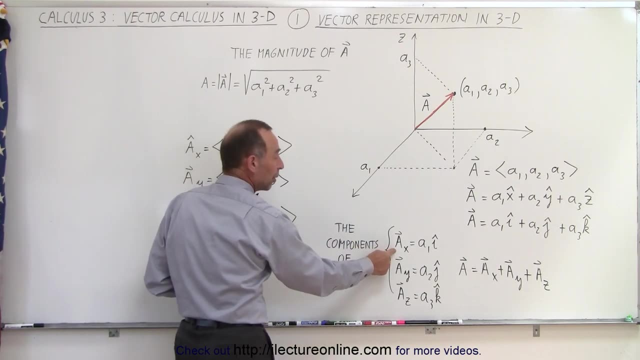 and z unit vectors. we can use i, j and k unit vectors. Now, the components of the vector a are vectors in themselves. this is how you define the three components: the component of the vector a in the x-direction. the component of vector a in the y-direction. the component of vector a in the z-direction. notice these.